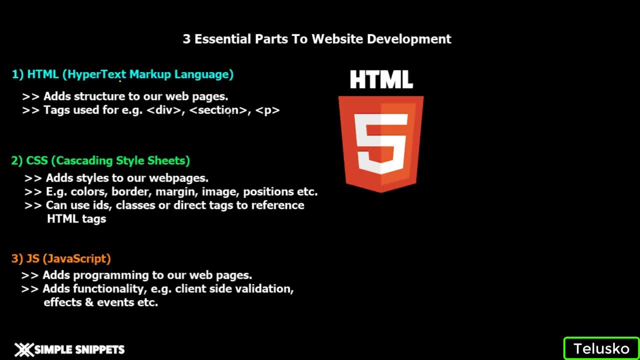 language, but it is used just to give structure to our web document or website. The next thing that comes here is CSS, which is cascading style sheets. It enhances the HTML by adding styles to our web pages, For example color border margin. 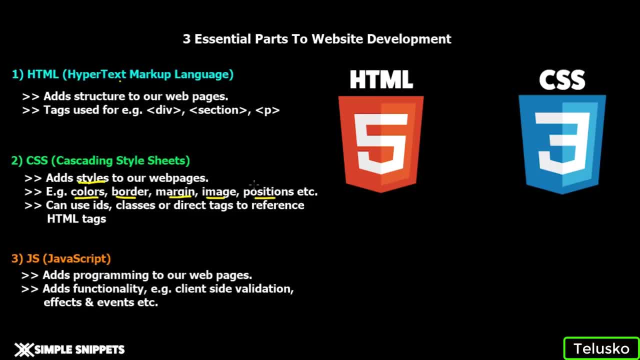 image positions, et cetera, And all these things can be handled in a separate file, which is cascading style sheets, or it can also be embedded in the same HTML file. There are two, three different ways in which we can use this cascading style sheets, but then 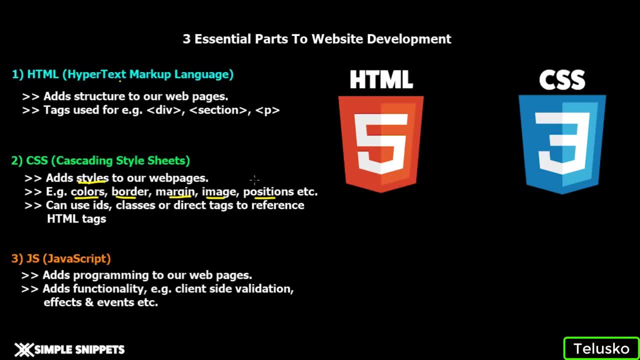 you get the idea right. In order to add certain design aspects and add certain styles, we use the CSS And lastly, the third part, that is, JavaScript, which actually adds programming to our web pages. So, using HTML and CSS, you can definitely develop a complete website. 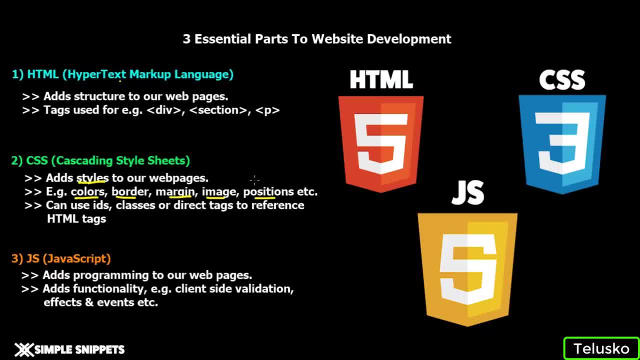 but then to add certain functionality. for example, if you have a button, when you click on that button, something should happen right, So that function can be added by using JavaScript. or let's say you have a form and you type in your name, and instead of name you type: 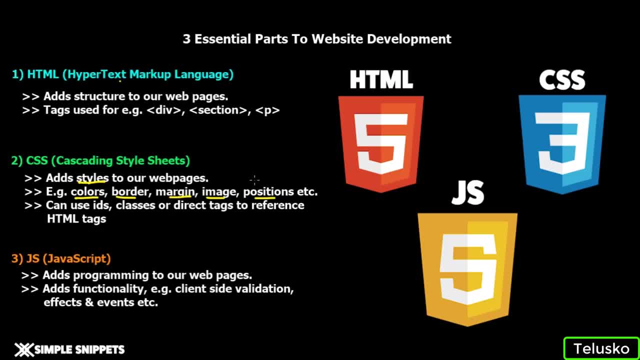 in some number. So you want to perform validations that you cannot enter number in your name section, right? So those kinds of functionalities on the client side can be performed using JavaScript. So when we combine these three things we get a complete client side website which has proper structure by HTML, which has styles. 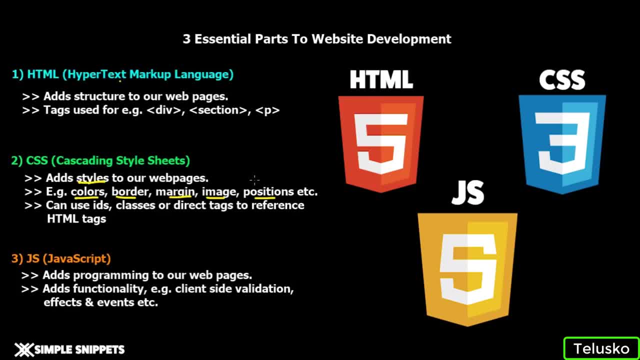 which is added by cascading style sheets, CSS, and which also has client side functionalities like validations, effects, events, et cetera, using JavaScript. Now the question arises: how does JavaScript interact with HTML document? Now, JavaScript is a programming language. 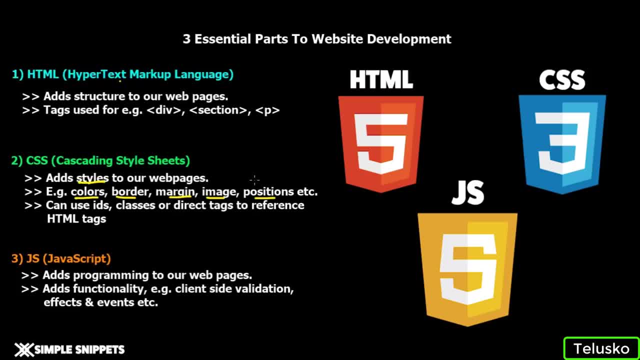 right, It is a scripting language which is embedded in the HTML document itself, or you can have a separate file, which we'll see in further videos. But then the question that arises is: how does JavaScript understand the HTML markup language? So this is where that document object model comes into picture. So let's take a look at. 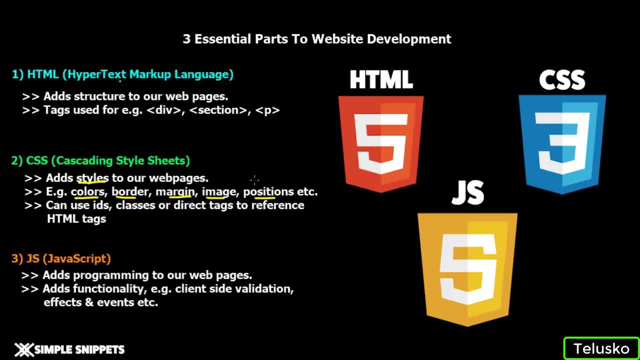 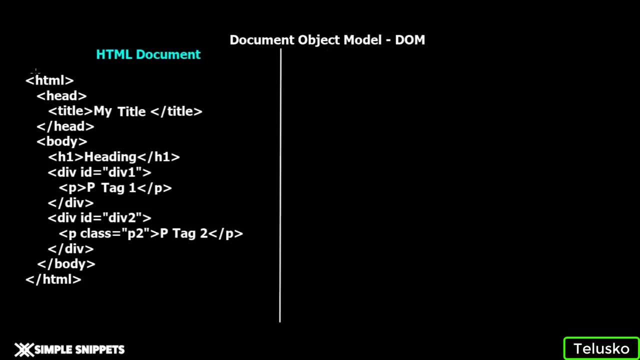 a typical HTML document and let's see a little bit of HTML markup language. Okay, So, as you can see, on the left side we have a HTML document And if you have even 1% of HTML knowledge, which is the prerequisite of this entire course, you can definitely understand this, because 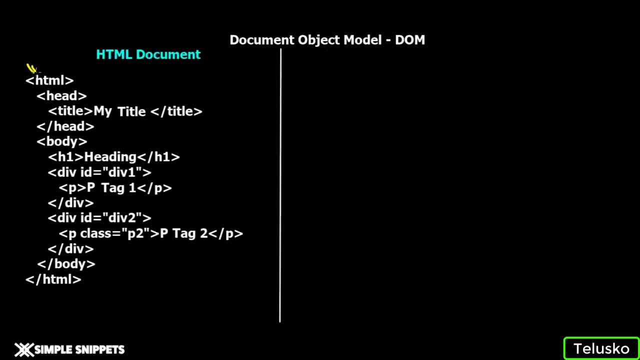 it is a very basic HTML document. So we have our HTML tag over here. So opening HTML and closing HTML, Then inside that we have head tag and then head tag closes. We also have body tag opening and body tag closing. Now inside the head we have our title tag and then we have certain. 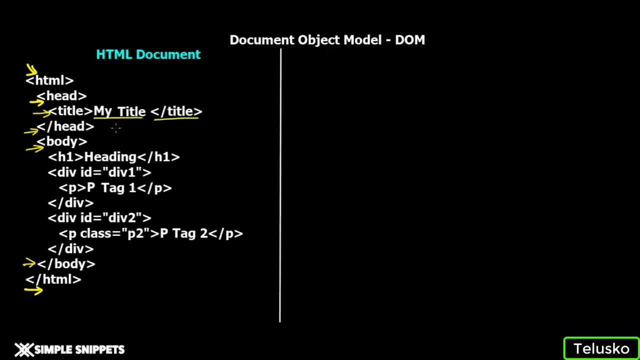 text, which is my title and the title that closes over here. Similarly, inside the body, we have heading tag H1.. We have one division with ID div one, We have another division with ID div two and inside those individual divisions we have paragraph tags. Okay, Now. 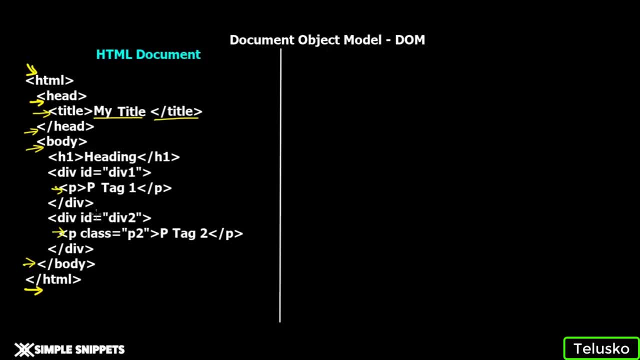 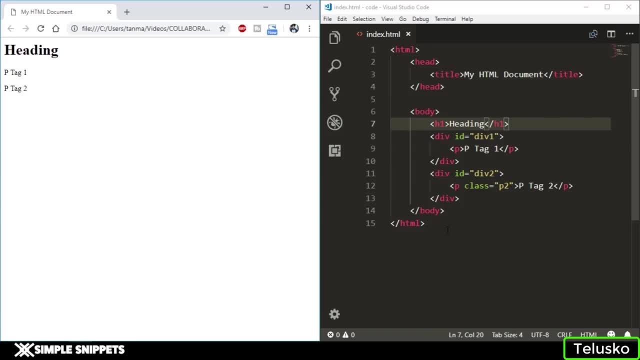 this is very basic, In fact. let me just actually show you the actual code, and we'll also see this code on the browser- How the web document looks. Okay, so, as you can see, on the right hand side we have the actual HTML code, And this is Visual Studio code editor. We are going to be using this. 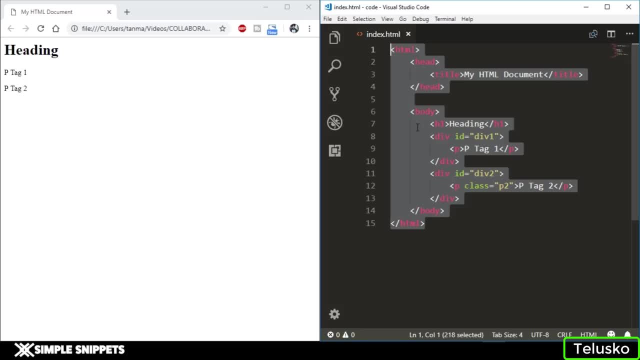 I'll talk about this in next video when we actually start off typing with the code. but, as you can see, we have our indexed HTML file and the same file is actually running on the browser. You can see file users and then the entire directory And, as you can see, we have 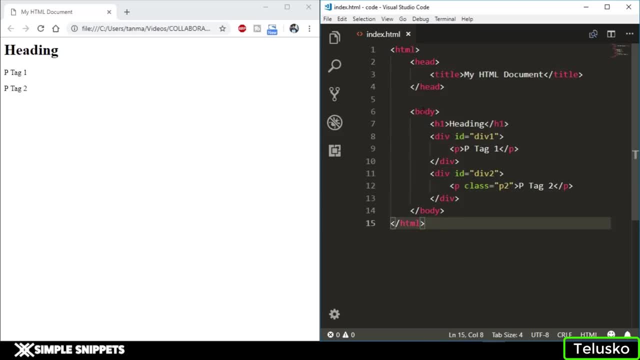 our title, my HTML document. Yeah, yeah, Sogon that title. Okay, inside the body we have our first heading h1, so you can see that heading is written. so this is a text. then we have individual two divisions, which of course cannot be seen, but inside those we have. 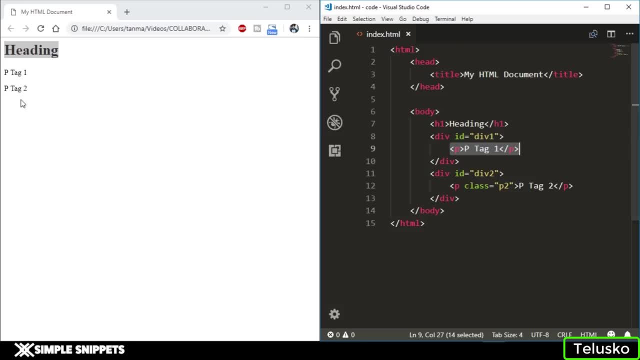 paragraphs and the first paragraph, we have p tag 1, so that's visible over here, and p tag 2, so this is visually what i wanted to show you. now let's get back to the digital blackboard again. okay, so now that you've seen the actual html web page load on the browser. coming back to our original, 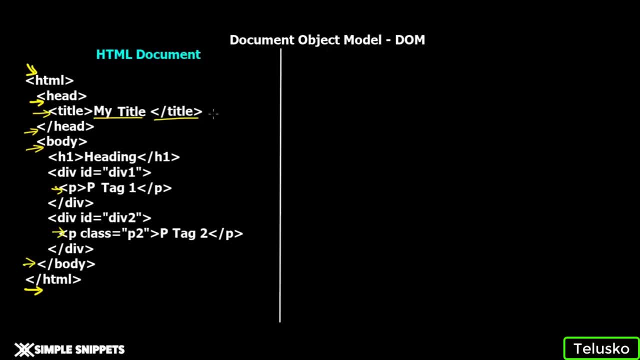 question: how does javascript understand this html document? so this is where that document object model comes into picture, and let me show you that dom entire model. okay, so what happens is when the html document is loaded in the browser corresponding to that document, another representation of that document is created, which is known as the document object model, aka dom. now this jsv represents. 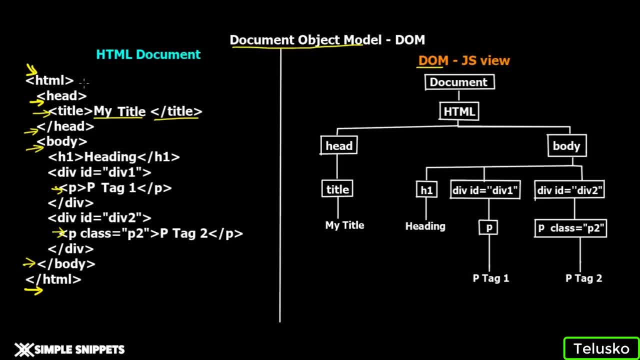 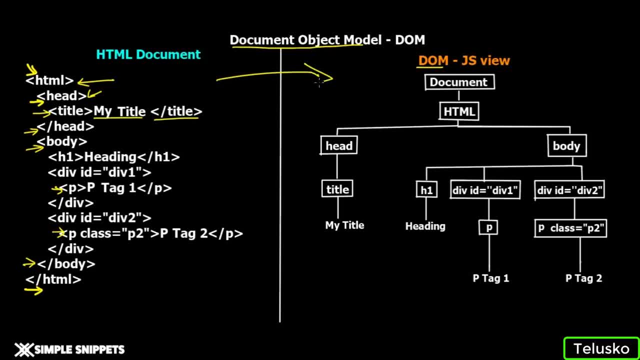 and, corresponding to this, we have another representation, which is the dom. so that's why it's a document and each of these tags are represented as objects. so that's why document object and since there is a hierarchy, you can see that the entire html document comprises of a. 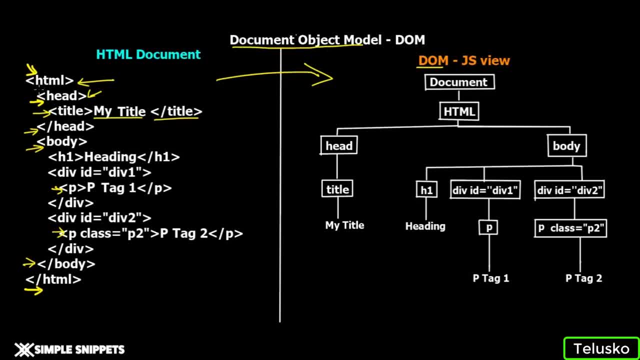 hierarchy right. we have html, which is the top node. inside that we have head and body. inside the head we have title and then inside the body we have again h1, first division and second division. so there is a proper hierarchy right. we also saw that in the code indentation. so similarly the same hierarchy is also created over here in the 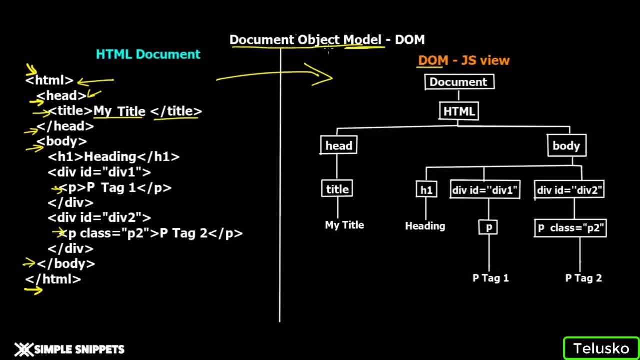 document object model, and hence the term model, so comprising of three words. document object model, is basically just a representation of the same html document in a different format. now, the reason why we require a different format is because javascript is a document object model, and so the javascript can easily interpret this format. javascript cannot understand this tags, but javascript can easily. 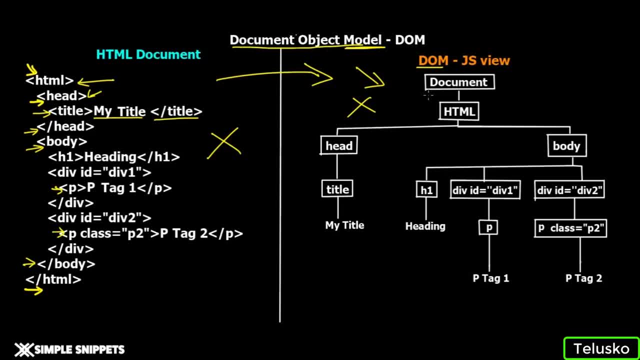 understand these objects. so this is where javascript can now actually use these objects to manipulate their attributes, since both these things are one and the same thing, so there is no separate document. it's just a different way of representing. javascript can now access each of these objects using different functions, which we will, of course, see in future videos- and then you can manipulate. 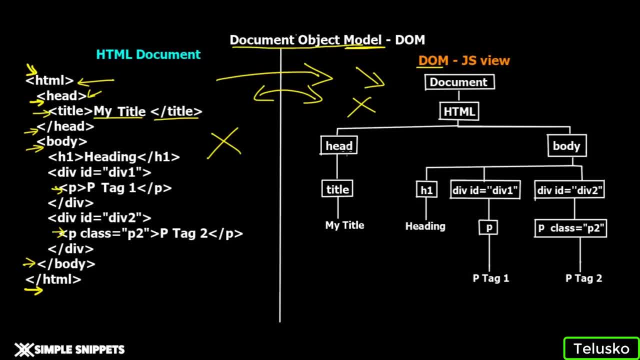 each of the attributes of these objects. for example, if you want to change the text inside the title, you can easily access this title object in javascript by accessing the document object model and then you can change the text inside the title. similarly, you can change the size, you can add color, you can add background to heading tag. 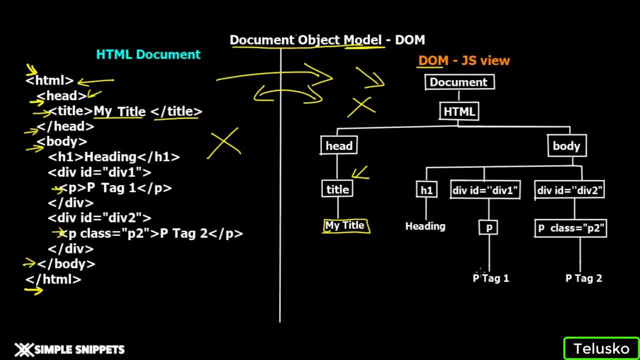 to division, to paragraph, you can change the text, you can hide the text, you can animate the text and you can do everything on this document object model using javascript. so the way it works is javascript looks at this document object model in terms of nodes. okay, so the concept of nodes is used over here and there are many nodes, but 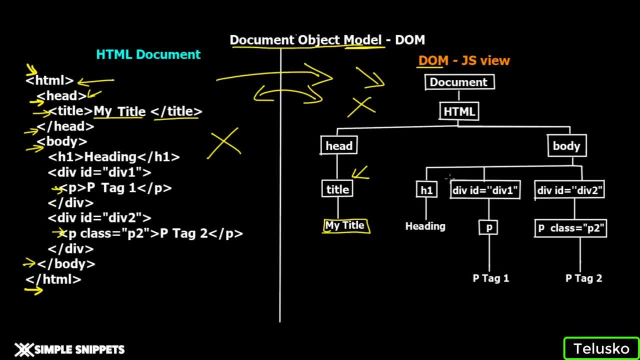 primarily, we are going to be looking at three different types of nodes, so let me just show you what these nodes are. so these are the three different types of nodes. number one is element node, so this is number one. number two is attribute node- this is number two. and number three is 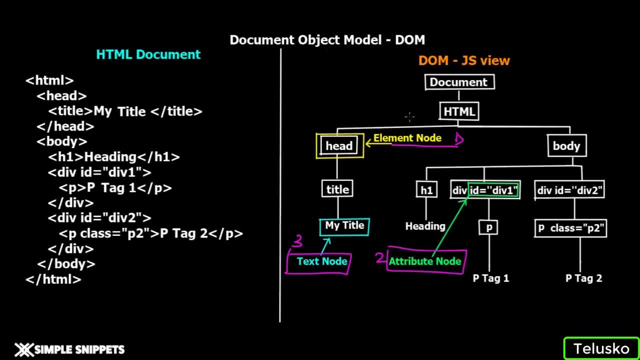 text node. so again, a little bit of hierarchy is going on over here. you can see that at the top level we have the element that is the tag itself, right? so the head tag, which is the tag over here in html format, is represented as an object over here. so everything in rectangular. 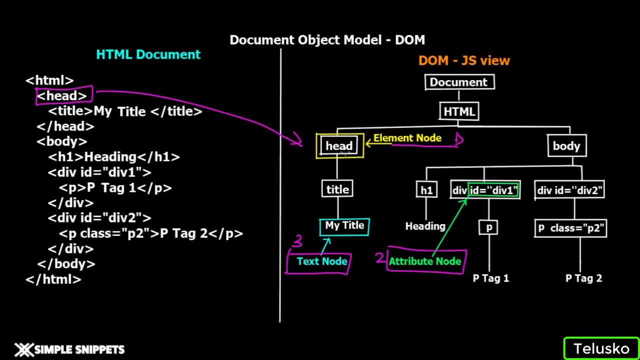 boxes is represented as an object. and for those who don't know object oriented programming or who have never even studied object oriented programming, basically your object is something which has an attribute as well as a method or function which can operate on that attribute. even though it sounds vague, you will understand it when we actually go ahead in the programming part. so 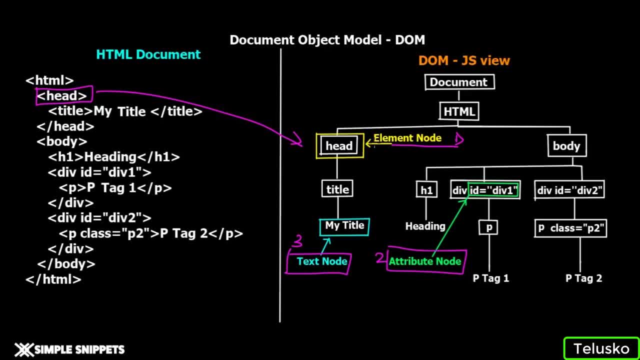 don't worry about that. so yes, this yellow box is the element node. the next in hierarchy is the attribute node. so now you can see that in the html form this division has a id of div1. right, we have given this id div1, so this id is basically the attribute of that division. even in html we call: 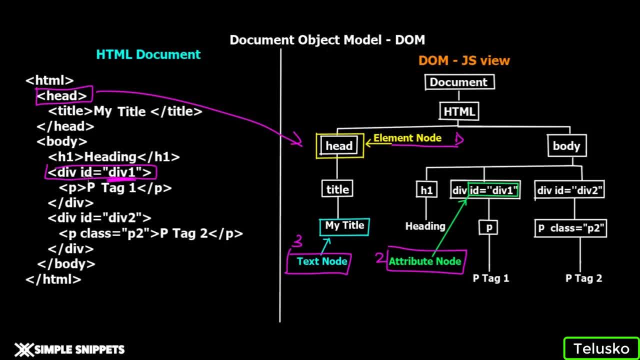 it as attribute, right? we have id, we have class, we can add style and so on and so forth. so these are the attributes. so this attribute node corresponds to this id and using this attribute node, javascript can actually do that, so we can add style and so on and so forth. so these are the attributes. so 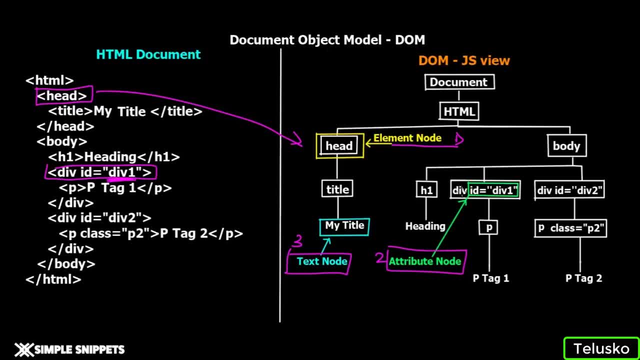 we want to access this type of gigs, build and build as的话 edges. so the Egg fields also write attributes inside of them. so we want to put the name order in docpy: 자 time поряд scprp, and then perform autocad outsay. a student type DB will start integrating and then in a moment, 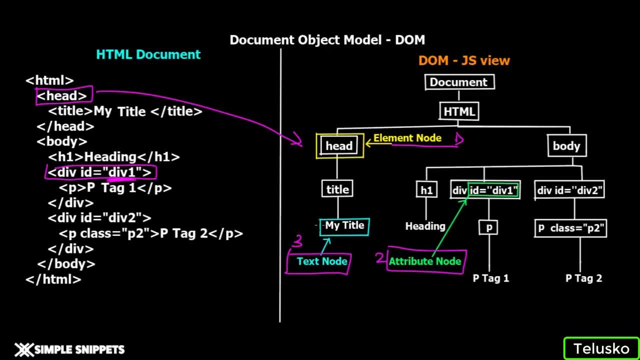 the last node is the text node, which is basically the content inside the element. so in this case, in this blue box, you can see that this, my title, is actually the txt inside the title tag. right, so this title is an element because it is a tag over here, but inside that tag you can see that we have 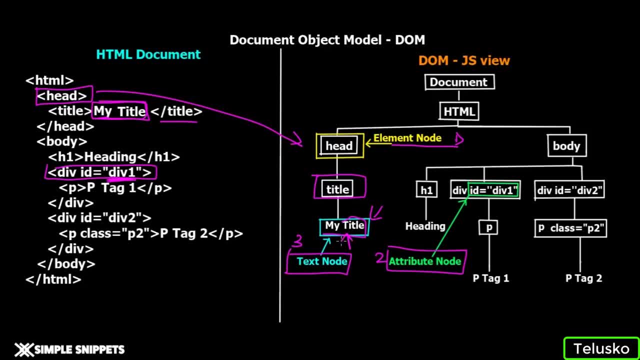 on some actual text. so that's why you can see this. my title is not actually inside a square box, because it is not an object, it is some attribute, or you can see it as a property. it is a value. right, so you can change this, my title, using javascript by accessing the text node. so these